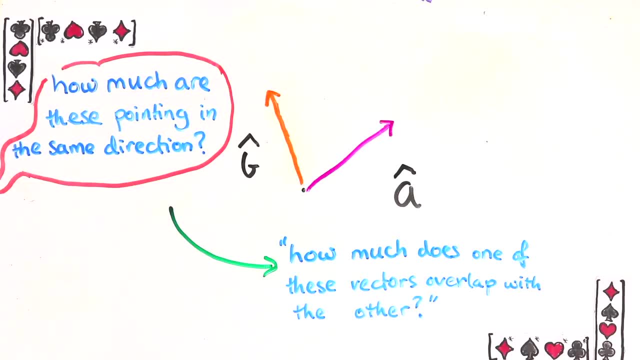 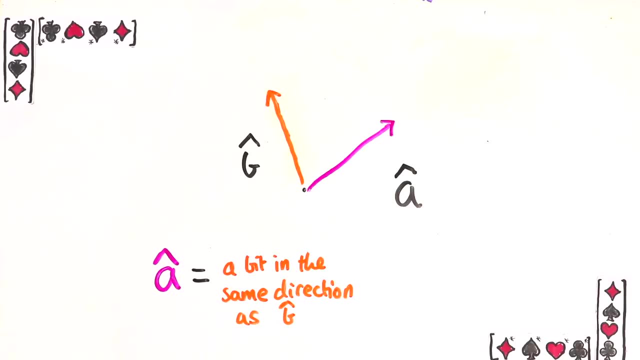 much does one of these vectors overlap with the other? What I mean is this: You can always write that a hat is a number. A hat is equal to some part in the direction of b, hat plus a bit that's completely perpendicular to the direction of b. Why Draw a little triangle like this and then have these two? 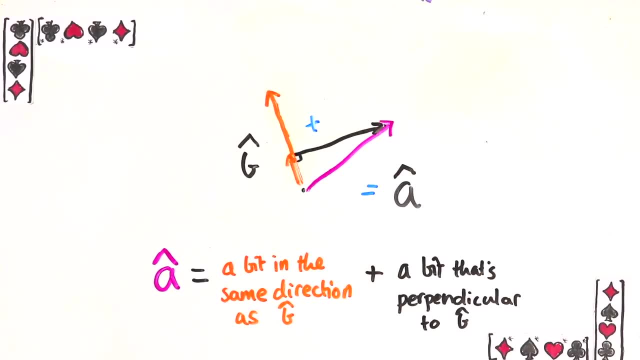 sides be vectors. They add up to the vector a hat, But this bit is in the same direction as the vector b hat, so you can write it as x times b hat, where x is some number. So a hat is equal to x times b hat plus a hat. 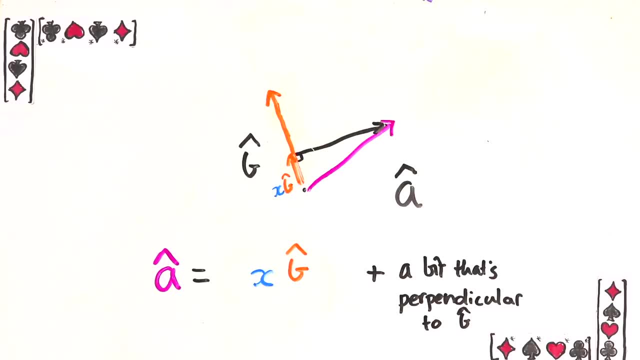 Plus something that's perpendicular to b hat. This number x seems like a good answer to our question, because it quantifies how much the a direction has of the b direction in it, which could be interpreted as the amount that they're pointing the same way. Still, that may not convince you, so let's do some. 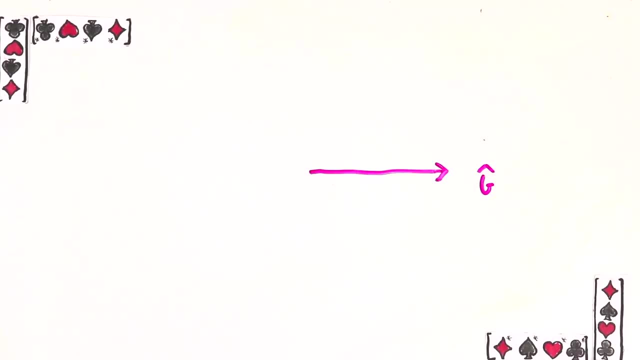 examples to help see it. Imagine they're pointing exactly the same way. Then a hat equals one times b hat, But then, as it rotates away, x gets smaller. This makes sense because they're less in the same direction. Then they're totally perpendicular and the number is zero Again. that makes 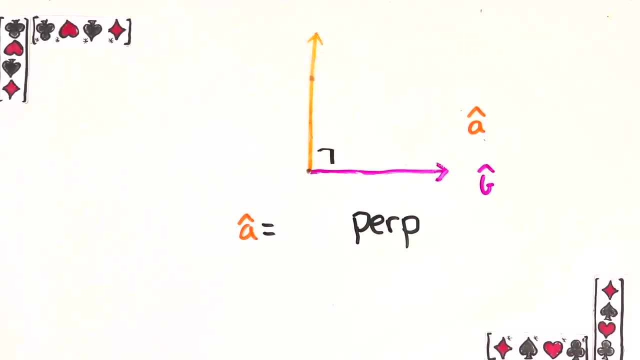 sense. But do you think that the number should get higher or lower if we keep rotating? Hopefully you said lower, since they're pointing even less in the same direction, But to check you get it. here's a question. Suppose that a and b are pointing in exactly opposite directions. What is x in this case? 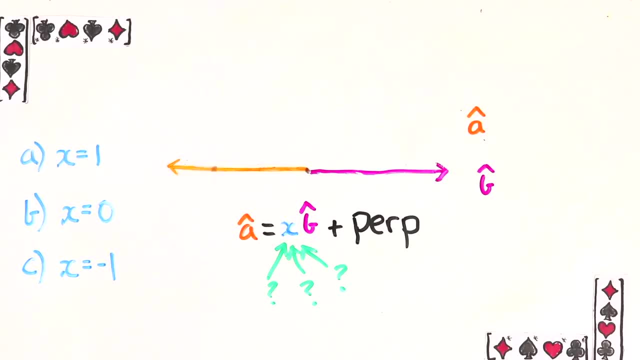 Here are the options, and I'd like you to actually pause the video and put your answer in the poll. Some of you might think that the answer to this is so obvious that there's no point actually doing it, But trust me, putting the effort in to answer it in the poll will help. 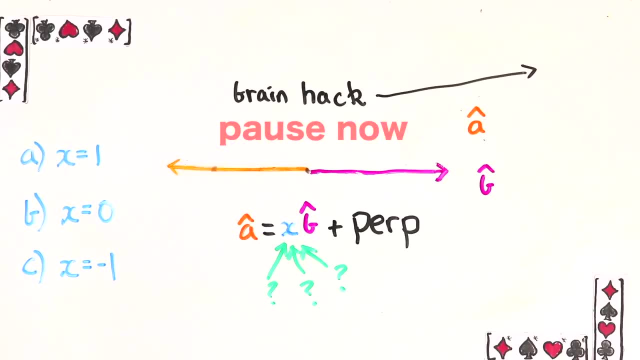 this stuff stick in your mind. Hopefully you found this video helpful. If you did, make sure to give it a thumbs up. I'll see you in the next one Bye 3. Hopefully you said the answer is minus 1, because a hat is now minus 1 times b hat. 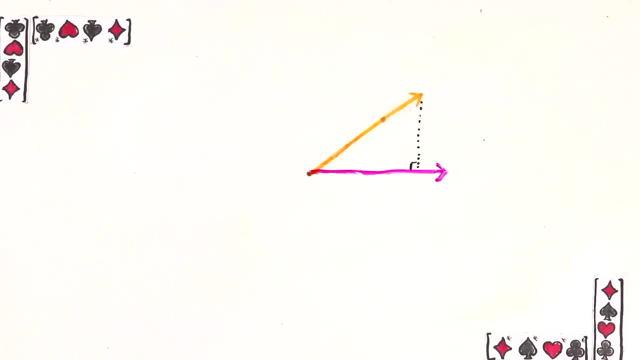 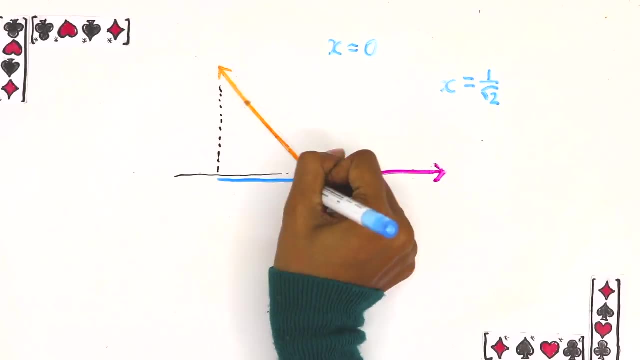 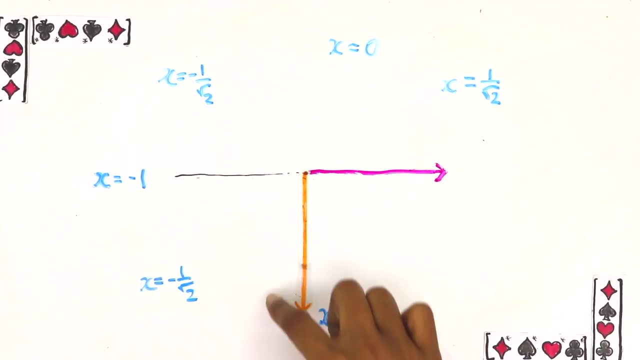 So great. this number x seems to be a good answer to our question, because the value of x decreases as a rotates away from b, and so it measures how much. they were pointing in the same way, But we need to figure out how to calculate it more easily. At this point, some of you 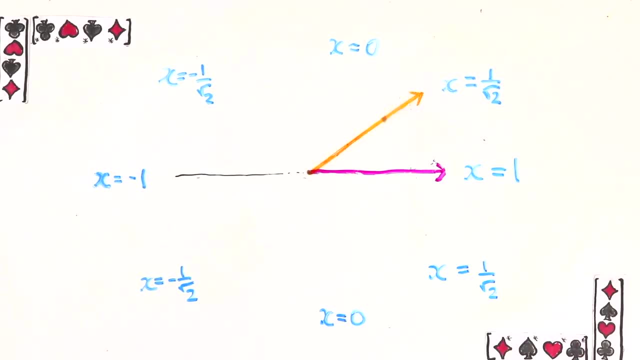 may have already started to feel a bit uneasy. You might be seeing some parallels between this thing that we're doing now and those unit circles with right angle triangles. they made you draw in school when you were younger. That's right. there's trigonometry involved. 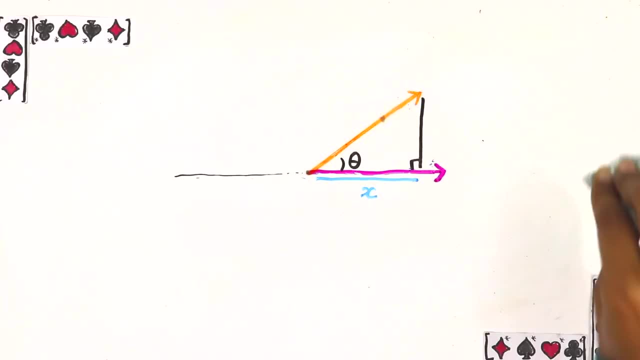 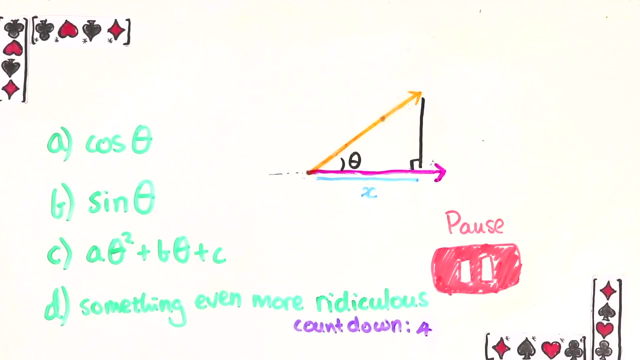 But okay, the trig is not so bad. So I want you to figure out which of these trig formulas is the number x in terms of the angle theta between a and b. Pause the video and figure it out. Hopefully you guys remembered something from those many hours in class talking about right. 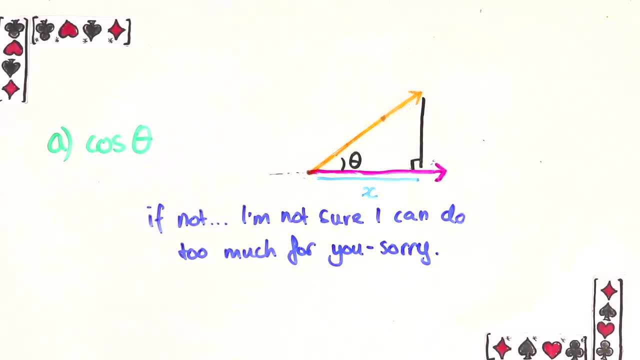 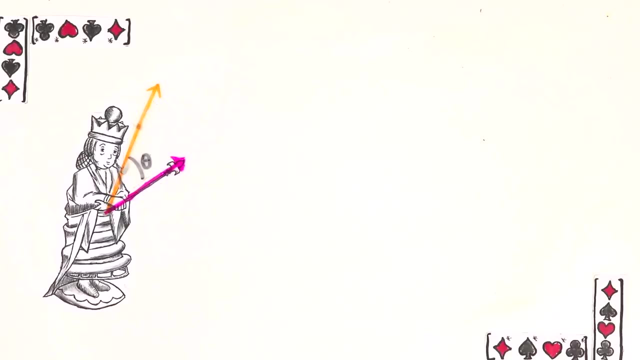 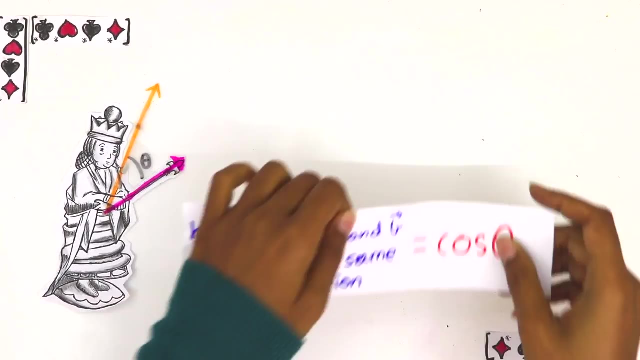 angle triangles and figured out that the answer is cos theta. So we have a nice answer to the question- how much do a and b point in the same direction? and even a nice formula for the answer: cos theta of the angle between them. But how does this relate to the dot problem? 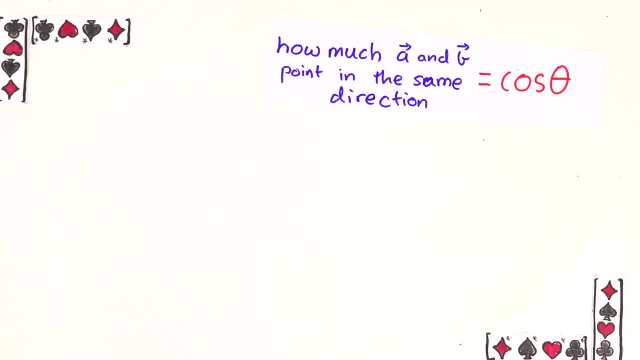 Let's take a look. The dot product is a function that takes any two vectors, a and b, of these lengths and gives you the amount that they're in the same direction, cos theta times their lengths. Why tack on the lengths? Doesn't that ruin the dot product's interpretation as being 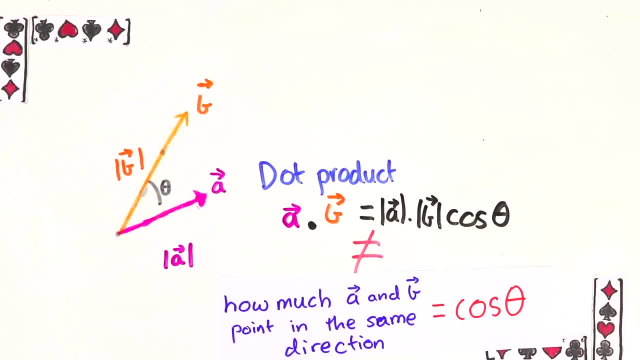 about how much vectors point the same way. Well, we added on because doing that makes the dot product a linear function, which I'll explain in a sec, and later on you'll see why that's such a boon. But right now I'm going to explain why, in an important situation, the dot product is. 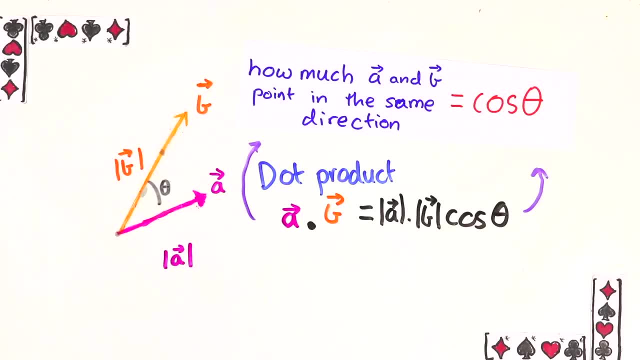 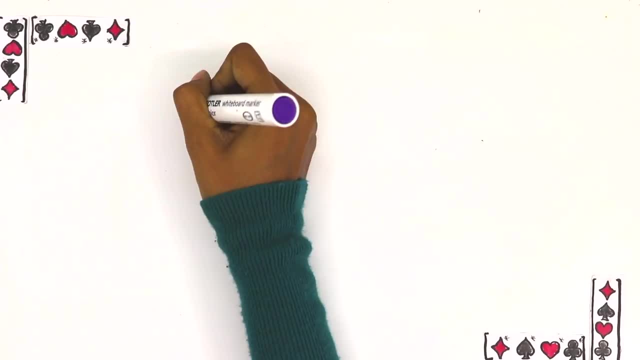 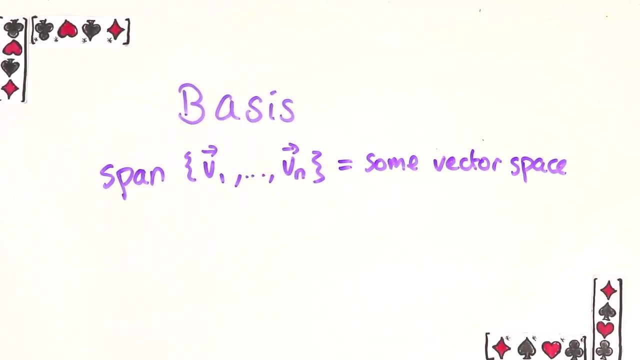 still very much about how much two vectors point the same way. That situation is when you have an orthonormal basis. As we know, a basis is just a bunch of vectors that span a vector space without redundancy. In other words, any vector can be written as a linear combination of the basis vectors. 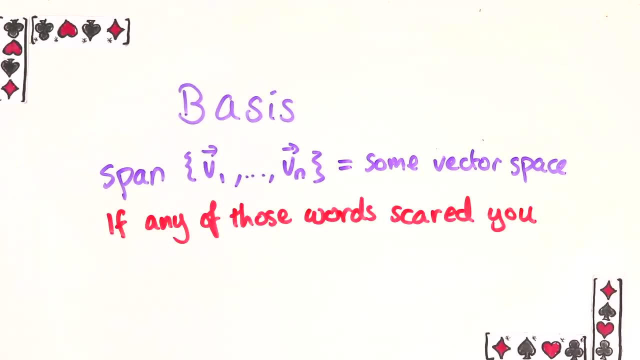 uniquely. If you're shaky on what any of those terms meant, you're wrong. The dot product is a linear combination of the basis vectors uniquely. If you're shaky on what any of those terms meant, you're wrong. The dot product is a linear combination of the basis vectors, uniquely.